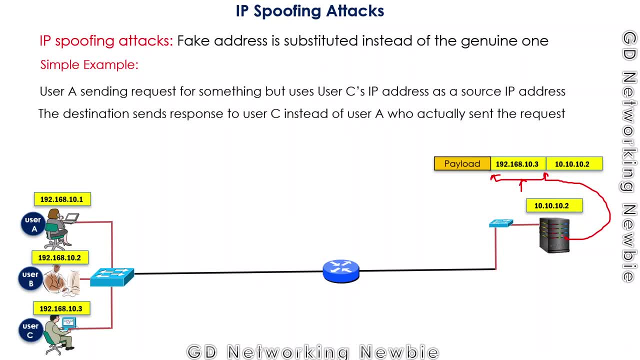 for that information. so this destination and response to that request will generate a packet along with the information. so let's say, this is the information which is needed and in the destination IP address, this machine will use the IP address of shock this one of this destination. so now the packet will be sent to this destination. 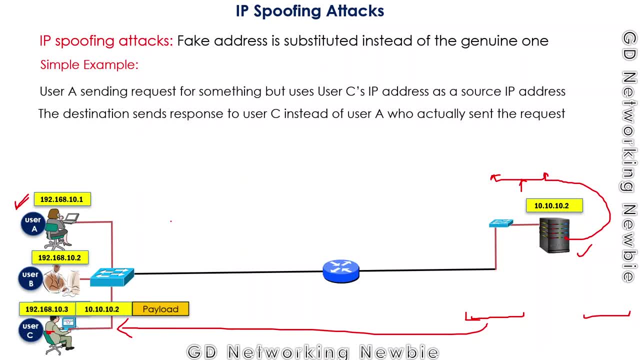 and state of the actual Center. so you can see here the Center has a Venezuela IP address and the purpose of this can be anything. for example, this user wants to make that IP address, have the standard, have at least spoofed the IP address and the locals of this can be anything. for example, this user wants to make a. 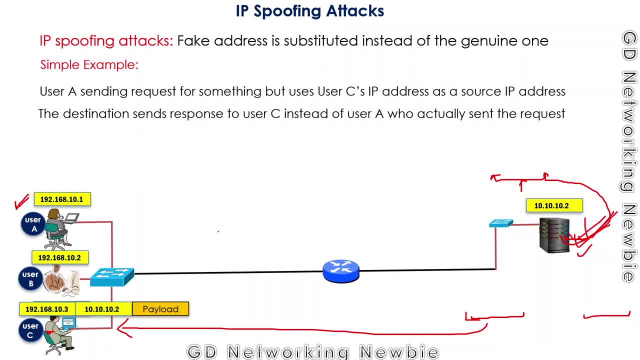 machine busy by using maybe different source IP address, so maybe at one time it can use the source IP address of this machine and then maybe this machine. in this way it can make this server busy or maybe there and that that user can use any IP address may be there and even if the in some of the cases there is no. 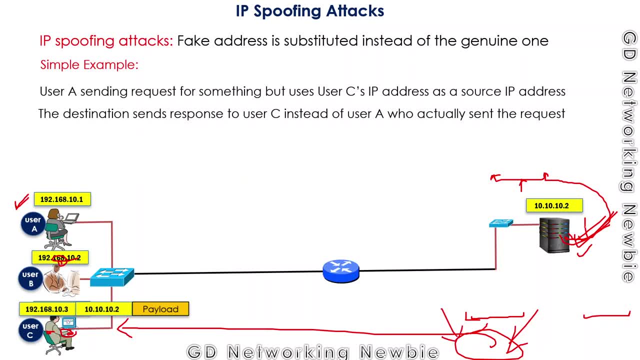 node on the network having that particular IP address. so in this way there can be any purpose of this user. so that can be like some bad guy, the network. so this is spoopy. now this user focus above the tercer can be anyone, not only on the same network, so this user actually can send. 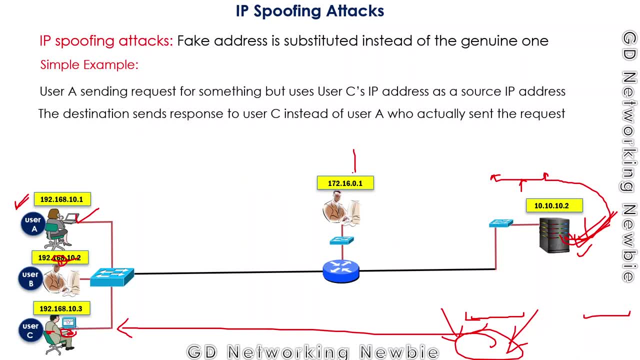 in the source IP address can send the IP address of this user. this user is somewhere else, so this request will be sent from this user to this server and or this computer and, in response, this server will respond back to this user having different ip address. so you can see, this is uh how this spoofing, ip spoofing attack can work. 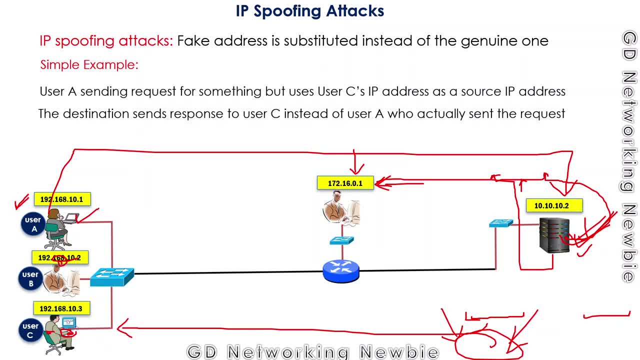 and this way actually there may be a state will come when this this server will be busy and this will not have any time to uh entertain the legitimate users. it means it will not be able to send a response to the legitimate users who are really needing the. 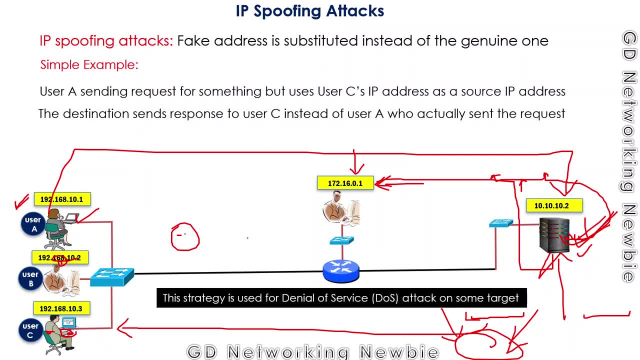 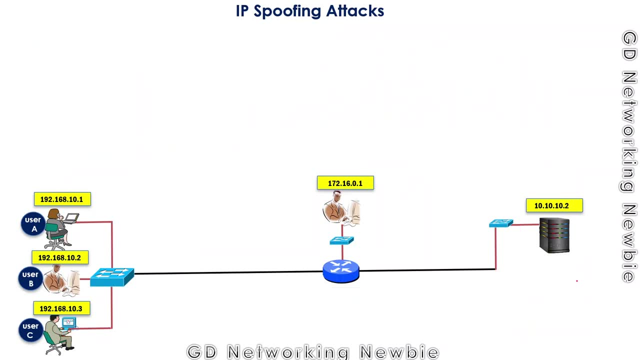 service. so this kind of attack is also known as a denial of service attack, because now this machine is in a state where it is- uh, it is denying the services to the legitimate users as well. and we can take one more example to understand it better. so let's suppose that user a, in this case this user, 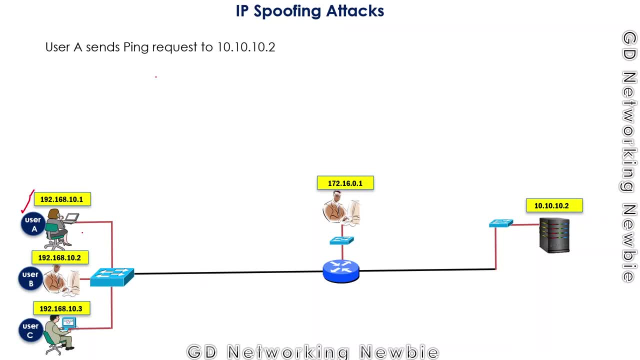 wants to is sending a ping request to some machine. that is this machine. so if you know that the ping request is sent to check the connectivity and the machine which is seeing the ping request, that machine has to send a reply and that is known as a big reply. so that has to send a reply. so it means 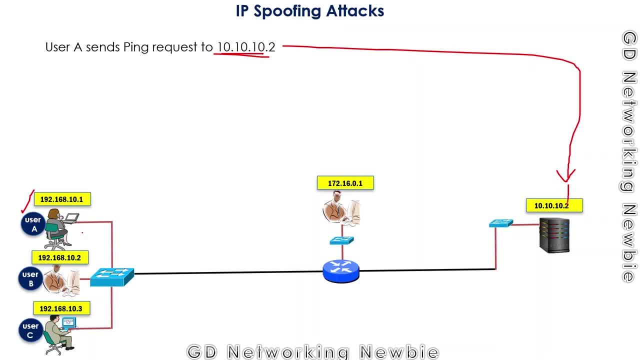 this user is sending the ping request to this one and the same user is going to send the ping request to the second machine, that's B this address, and the same user A is going to send the ping request to user C as well. so it means the user A is sending ping request to this one, to this one and to this one. 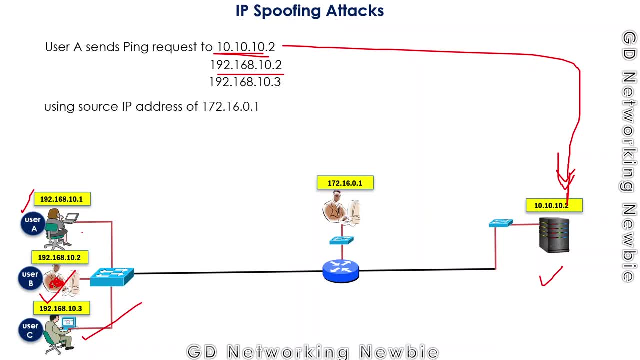 as well. but what happens in the source IP address? so for ping request it has to generate a packet. in that packet it will have a destination IP address and the source IP address. so in the destination IP address it is using the IP address of this machine, of this machine, of this machine in this machine. 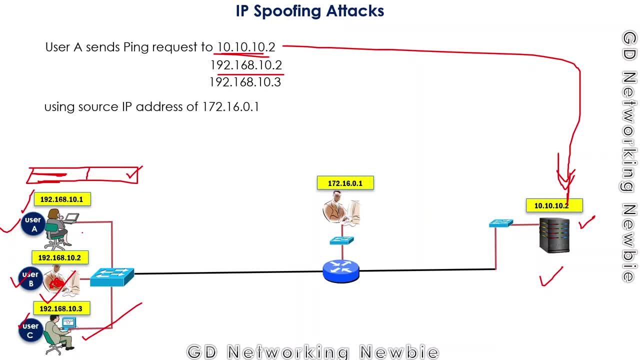 but in the source IP address. maybe if this user will use the IP address of this computer now what will happen? so in this case, all these machines, all these computers were receiving the ping request. they will send a reply back to this computer, see, to this machine. these all will send a ping reply message to all these. 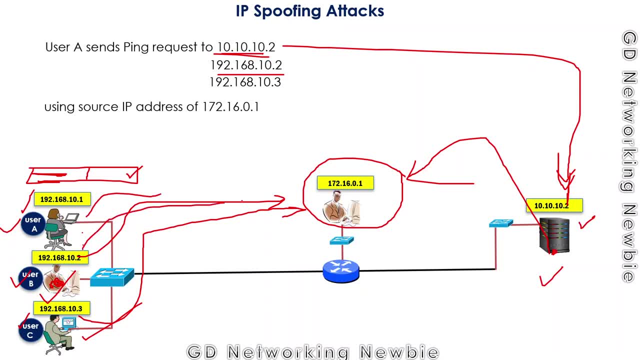 machines in this way. so sorry, so this one. so in this way, actually this user, so let's say this user has made busy all the computers where. so let me. so this user actually has somehow attacked this computer by utilizing other computer. so this is also a denial of service attack. and it can use, so distribute the.